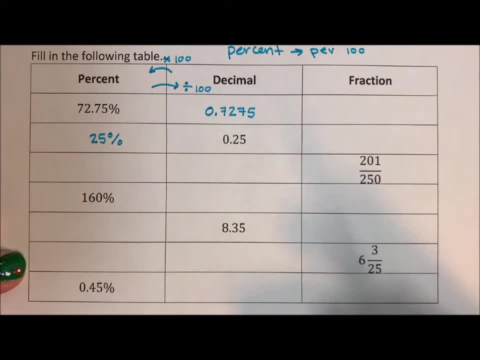 It's a way of dealing with small numbers in an easier fashion. So to go from here to here, we divide by 100.. 160 divided by 100 is 1.6.. 8.35 times 100 is 835 percent. 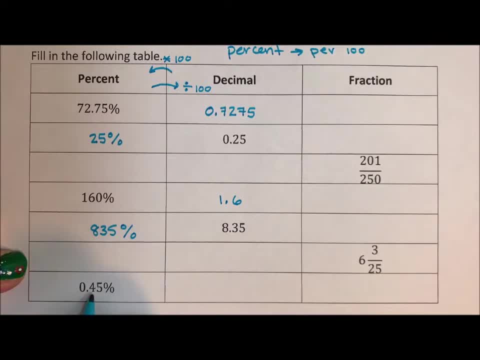 Nothing is here, And this is the one that always trips students up, because they don't want the decimal to be even smaller. But we are dividing, so we have 0.0045.. Okay, So there's nothing more we can do until we move these numbers over. 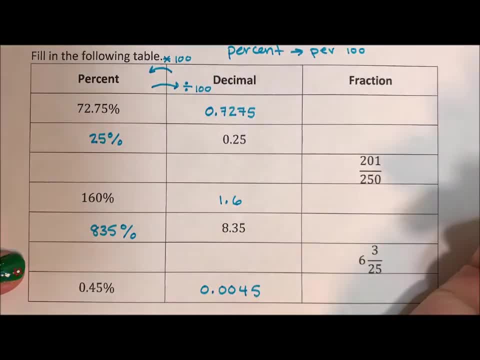 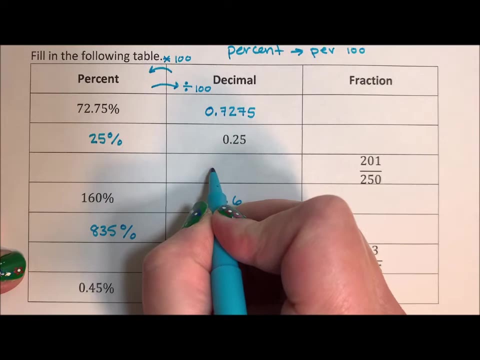 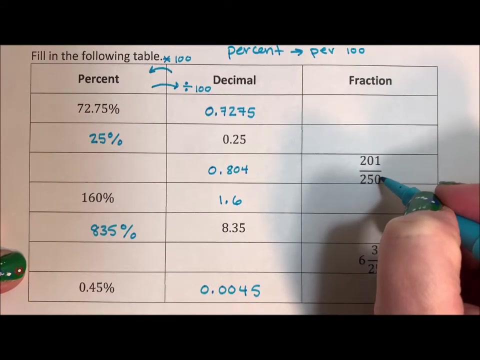 Okay To go from a fraction to a decimal. we just divide. So we could just throw this into a calculator And if we took a calculator out and said 201 divided by 250, we would just get 0.804.. Now if we're doing this without a calculator, 250 goes into 1,000 four times. 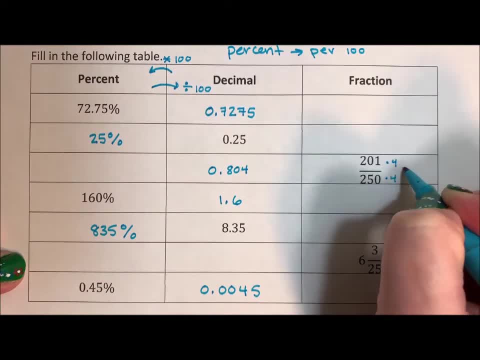 So if we multiplied the top and bottom by 4, we would get 804 over 1,000.. 1,000 is 3 zeros, so we move the decimal back three spots and we would get 0.804.. Here we could do the same thing. 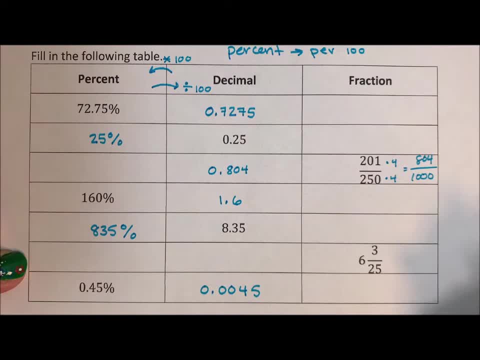 25 goes. there's 4 quarters and 100 and a dollar. So we multiply top and bottom by 4 to get 12. over 100 to get 6.12.. Or we could throw it into a calculator if you are using one. 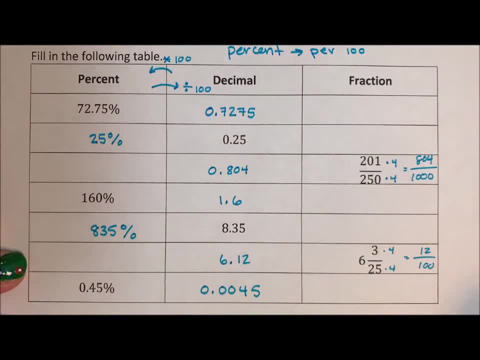 Depends on how you're being allowed to do this. So now we can multiply by 100 to get 80.4%. We can multiply by 100 to get 612%. Okay, Now the decimal. You take the number without the decimal point. 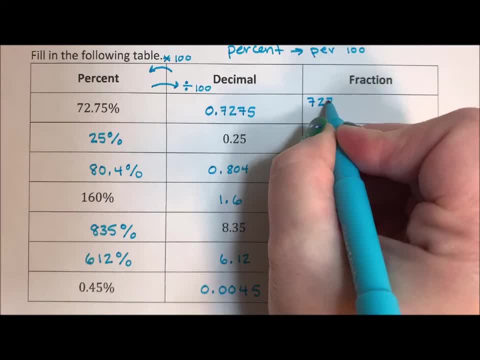 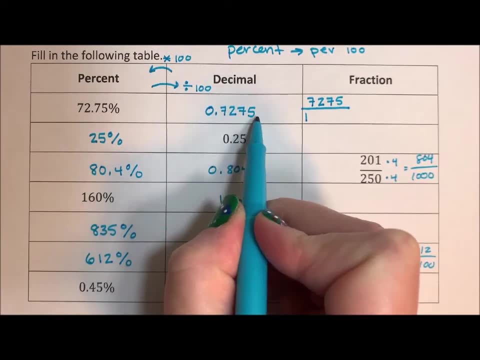 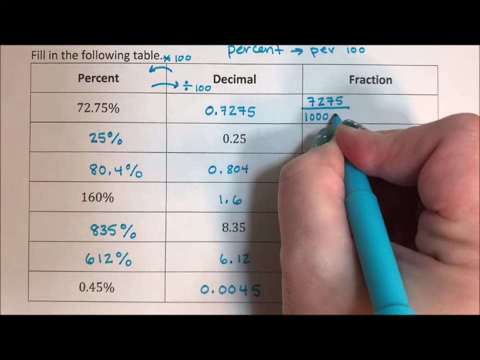 712.. 275.. And you put it over a 1 with the number of zeros, as there are numbers past that decimal point. So there are 1,, 2,, 3,, 4 numbers past the decimal point. So we do 1,, 2,, 3, 4 zeros. 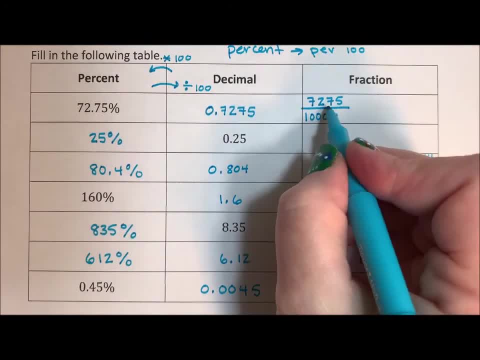 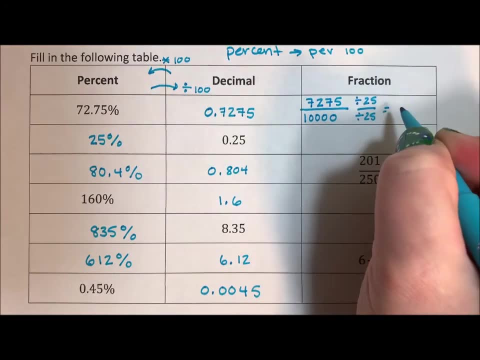 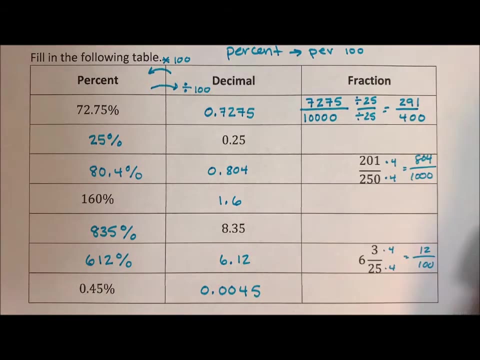 Now we have to reduce it. Well, 75 is the last two numbers means I can take a 25 out of top and bottom. If I divide top and bottom by 25, I get 291 over 400.. And since 291 is not divisible by 2 or 5,, 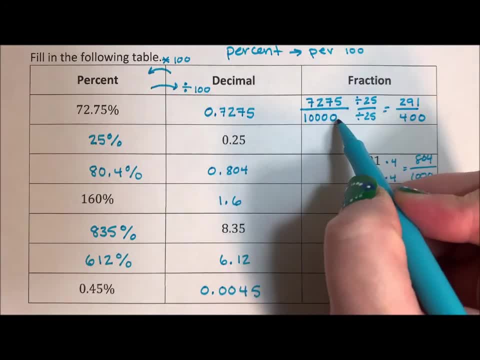 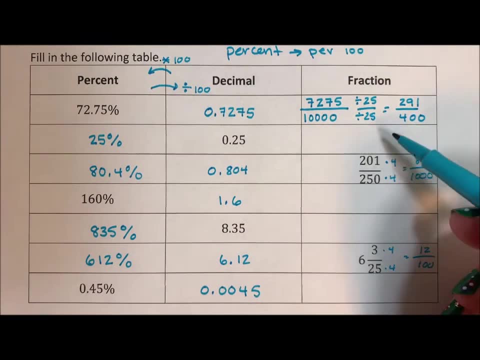 I am as reduced as I can get. The denominator is a power of 10, and 10 is only divisible by 2 or 5.. So when you're reducing these, you only have to look for 2s and 5s. 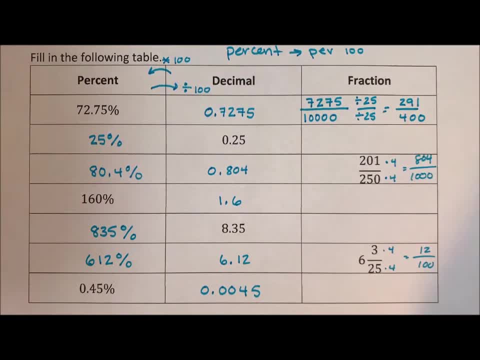 If it's not divisible by 2 or 5, you can't reduce it. So that's one nice thing. if you're doing this by hand, You're only checking if it's even or ending in 5. If it's not, you can't reduce it any further. 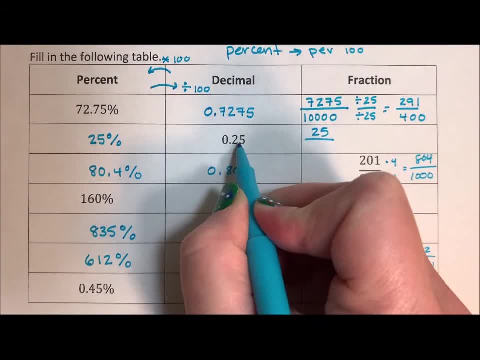 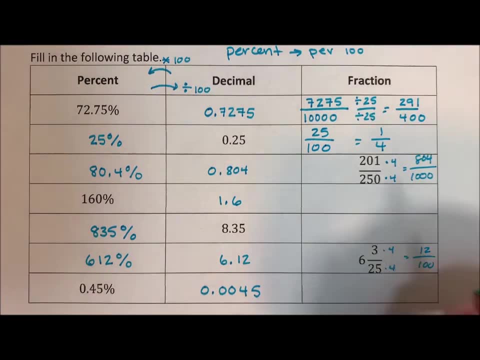 Okay, 25 has 2.. So over 100.. And I hope everyone knows that this is 1. fourth, because 25 is a quarter. Okay, So, noticing that this is 6 and a fraction, I'm just going to say 1 and 6 over 10.. 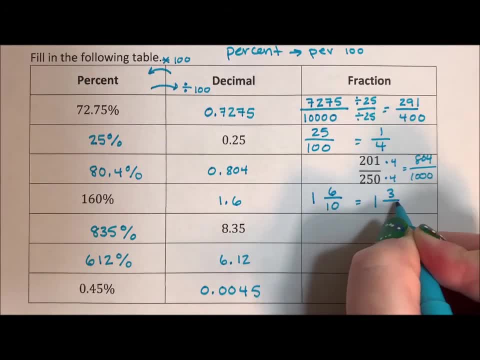 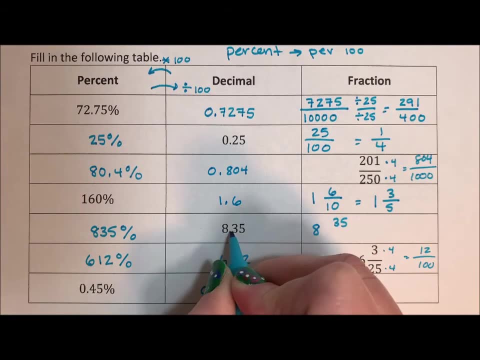 Which is 1 and 3. fifths, I can divide a 2 out of both of those 8 and 35. There are 2 decimal places, so 2 zeros. That ends in a 5.. So I can take a 5 out of top and bottom. 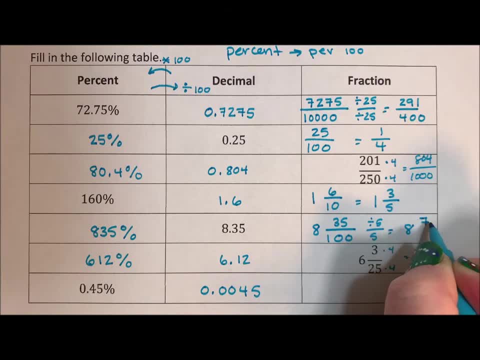 Which is 8 and 7 over 20.. Okay, So I'm going to put a 45.. 1,, 2,, 3,, 4.. That's 4 zeros. Remember I said there's a zero for every number after the decimal point. 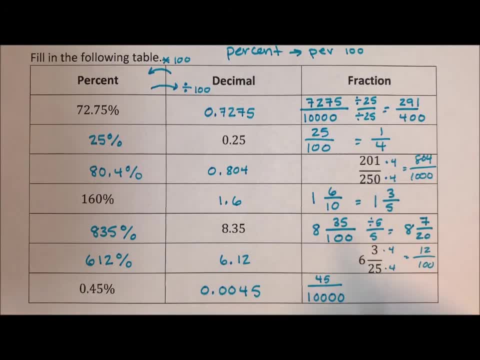 I didn't say non-zero number, I said every number. Okay, Divide top and bottom by 5. And I get 9 over 2,000.. And now we have filled out our full table. Alright, I hope you've enjoyed this video. 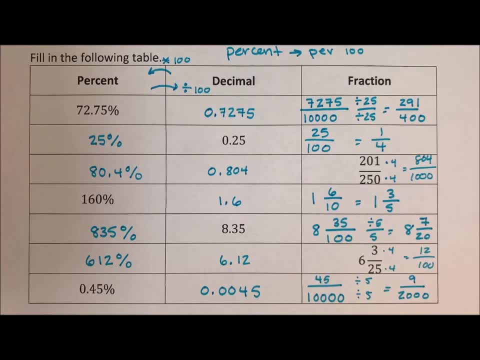 Please subscribe to my YouTube channel, Like my Facebook page, And I'll see you on the next video. Thanks,